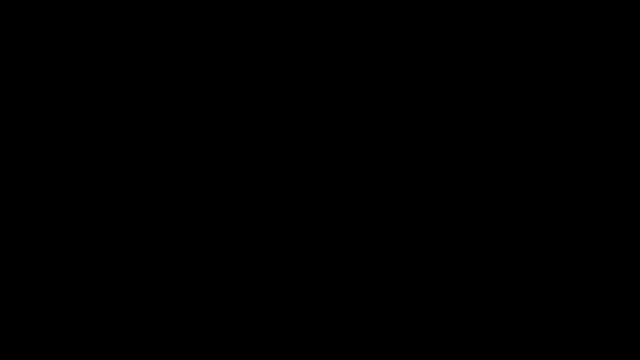 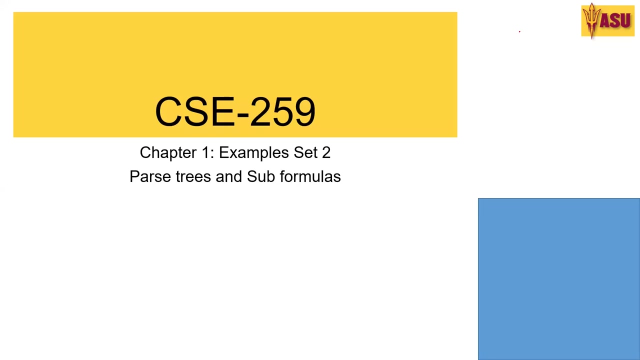 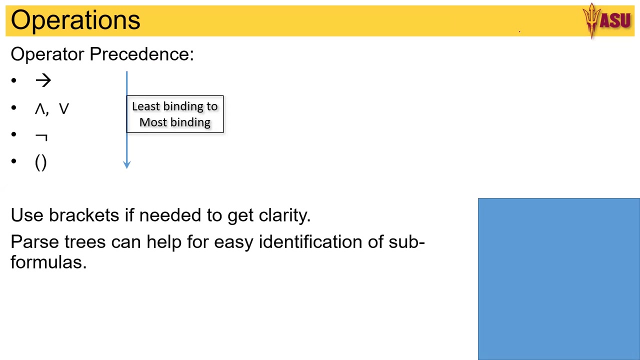 Hello and welcome to another session of recording for Example Set 2 of CSE 2.9 Chapter 1, Propositional Logic. In this set, we will see parse trees and subformulas. We will try to understand how to draw parse trees and how to decipher the subformulas of a given tree. The first most important thing as a recollection is we need to remember the operator precedence. So from the least to the most binding. Implication is the least binding. Then AND and OR have equal priority and NOT. And the most binding is the bracket. It will help to draw brackets around your formulas to get better clarity when we are writing out the formula. And parse trees do help with identification of subformulas. So if you are asked to identify subformulas, having a look at the parse tree would definitely help. 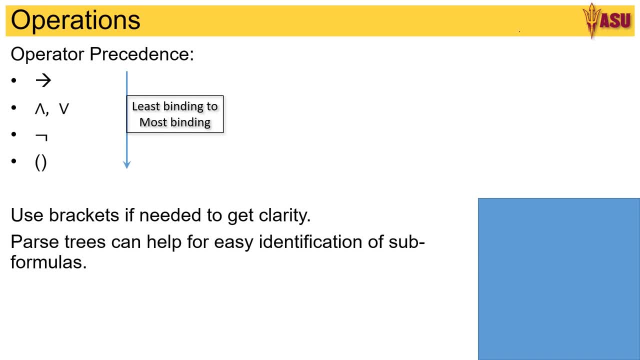 So let's see how do we get these brackets and how do we get to draw some parse trees. 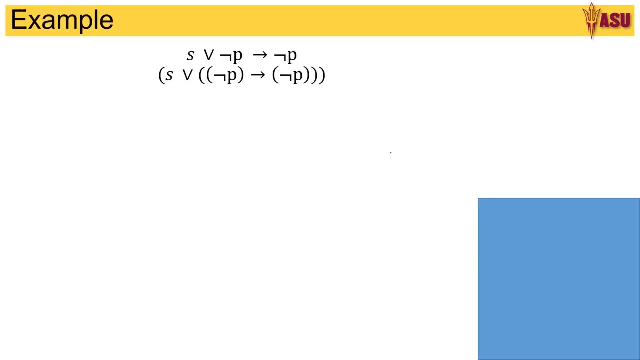 So let's take some examples here. Okay, so here are two formulas. One is s or NOT p implies NOT p and s or NOT p implies NOT p. Both are the same, but what's the difference? Okay, so let's take the first formula. We have s or NOT p implies NOT p. So the binding, if you remember, the most binding is a NOT because we don't have brackets over there and the least binding is an implication. So if I have to draw the... braces to make, have better clarity. So this is a NOT p. Then, the R has the next level of binding, it binds more tightly and the implication is the least binding, so that becomes this. 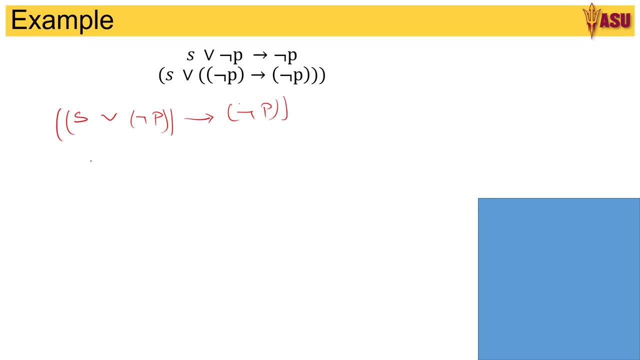 So what would the parse tree for this look like? So the topmost would be an arrow, that's implication, on one side of the implication is the R and for the R we have an S, the other side we have a NOT and P. The other side here we have NOT and P. So this is the parse tree for this, this is, we call this one, this is for formula 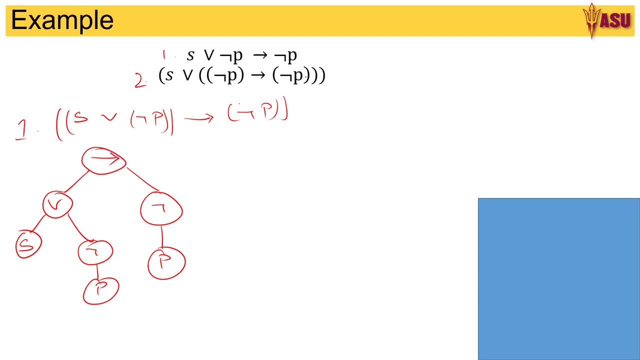 one and for two, what would be the parse tree for two then? What's the difference? So let's have a look at the brackets. So this is one. 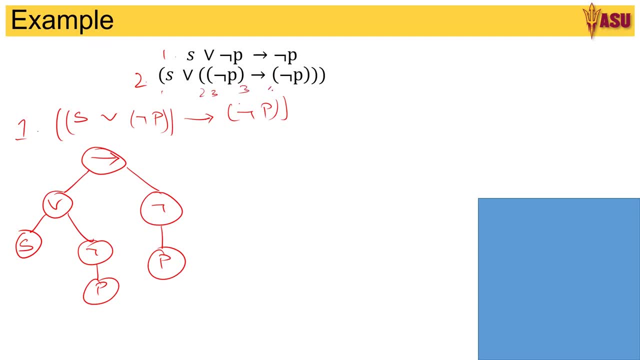 One, two, three, three, four, four, one. 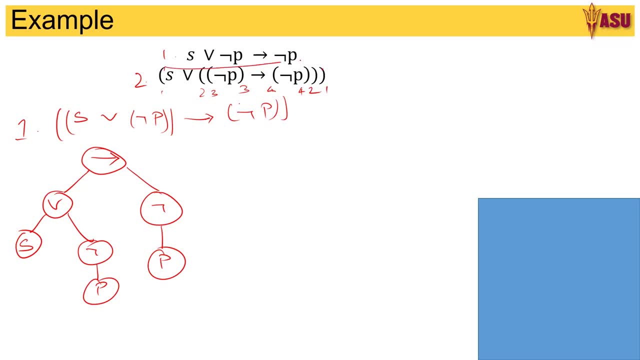 So this bracket corresponds to this, this bracket corresponds to this, this and this. So now if you see, the implication is not the highest priority here because of the brackets. So the parse tree for this would look like, let me draw it over here. R because R is the outmost operation, R has an S on one side and the other side is an implication and what are the other side of the implications is a NOT, P and the other side is an implication. So, in this case, the parse tree is just a NOT, P and the other side is a NOT. So, this are the two different subtrees for the formula we changed based on the braces that have been provided in the formula. 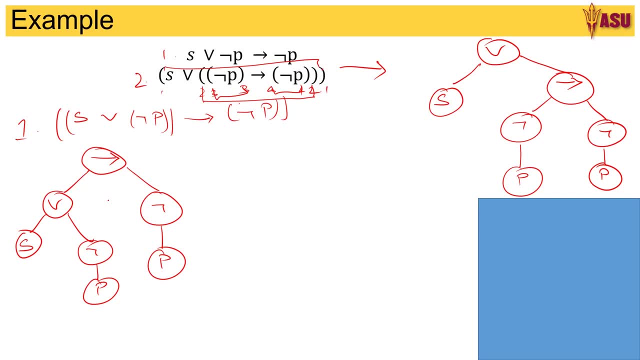 So it's very important to understand the braces in the formula. 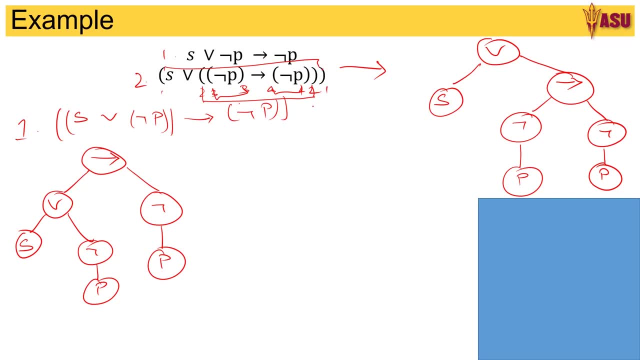 So now let's have a look at the subformulas that are there and how they would be different. 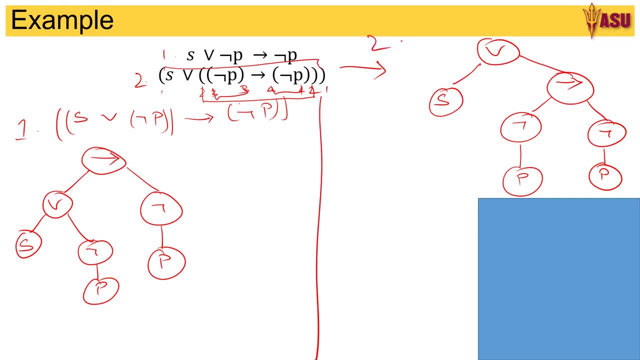 So let me separate this out here. This is for problem one and this case is for problem two. So here subformulas. So you have P. And then here. The other one is S. So that's the base tree. Then you have a not p. Not p, not p. Then you have a yes or not p. Not p and then you have the complete formula. 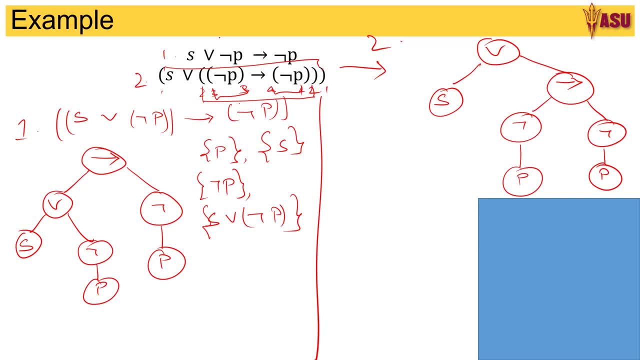 So these are the sub formulas for equation 1. 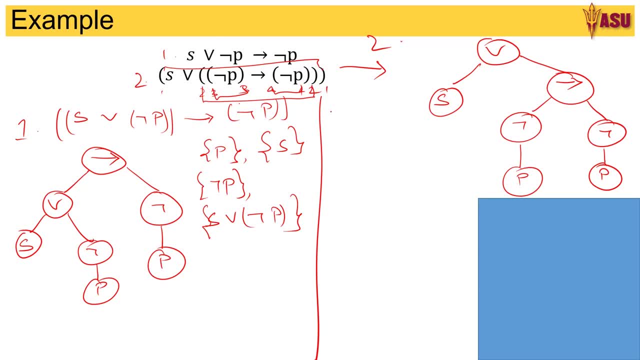 For equation 2, let's see what are there. Again you have S and p. You have a not p. Now if you see, we have not p implies not p. That's another sub formula. And 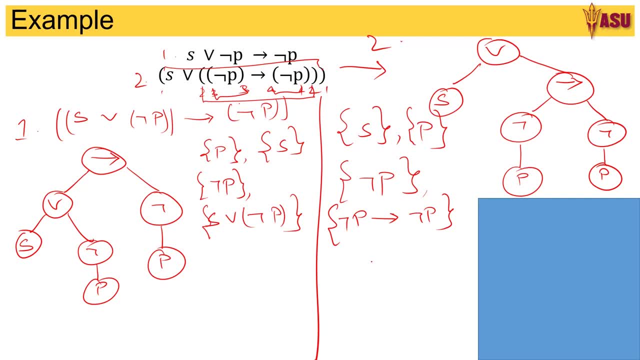 S or the rest of it becomes the actual formula. So these are our sub formulas. So you see there is a fundamental difference even in the sub formulas over here. I hope this gives clarity on how to use the braces to get a better understanding of the 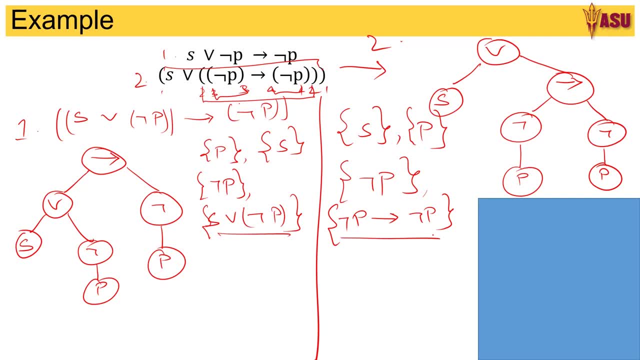 formula and how to draw the parse trees. 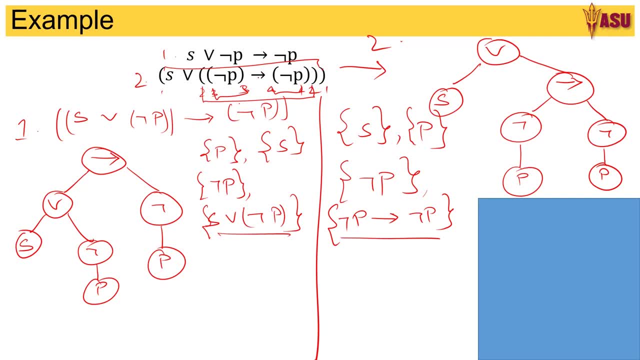 Don't forget the operator precedence. Implication has the least binding. Or and and have the next level of binding. 0 is more binding and the braces are the most tightly binding. 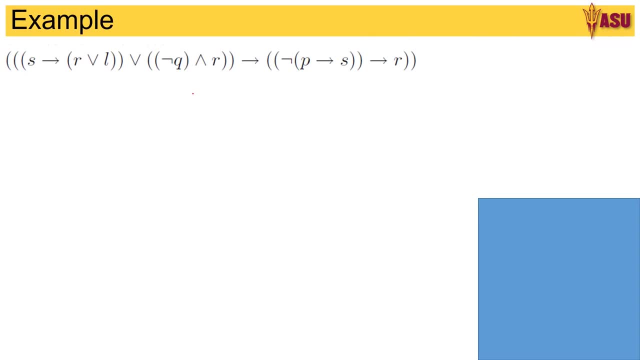 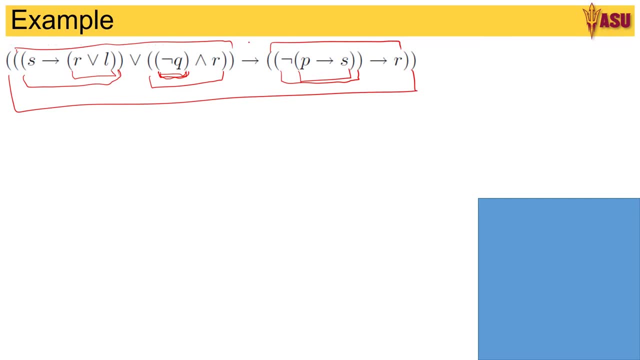 So you see that. Implication stands as the center of the entire tree. 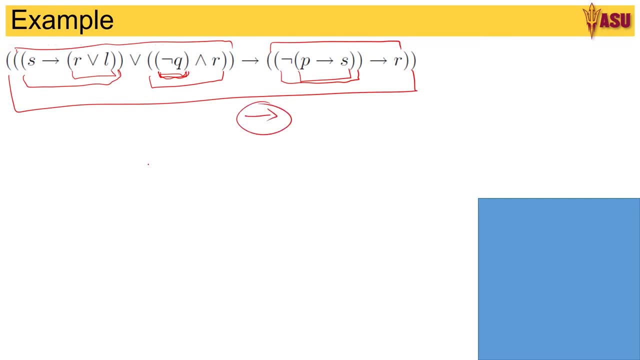 So the topmost is implication. 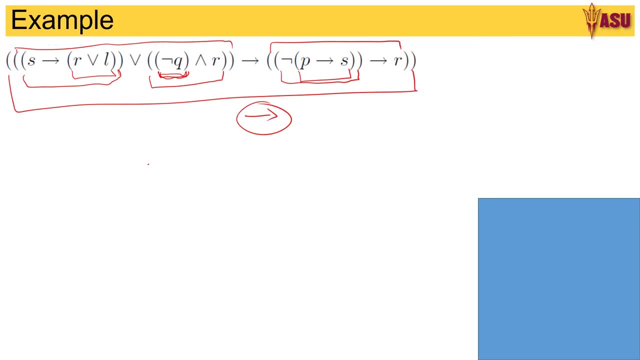 And given that all the braces are present in this formula, it makes it much easier to draw. Okay. Okay. 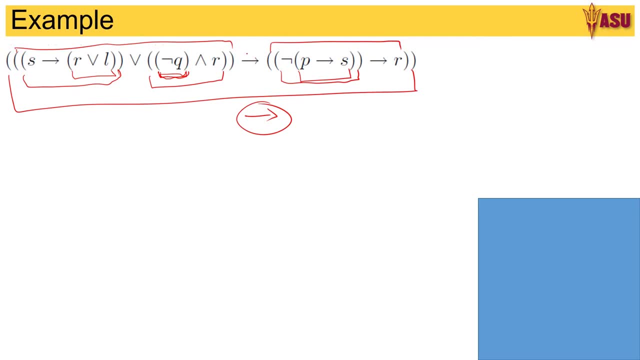 So I've drawn the implication and now let me take what is to the left of the implication. That is this entire formula. The center is an R. So I put an R. Now to the R, again I go to the left, I have an implication 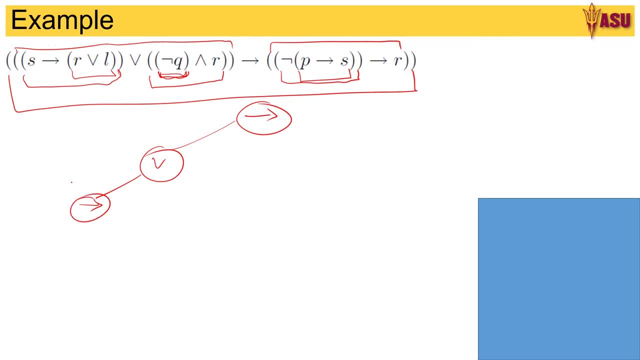 again to the left of the R. To the implication, the left of the implication is S. To the right is another R. For the R, I have a left is R and right is L. So that completes this formula. 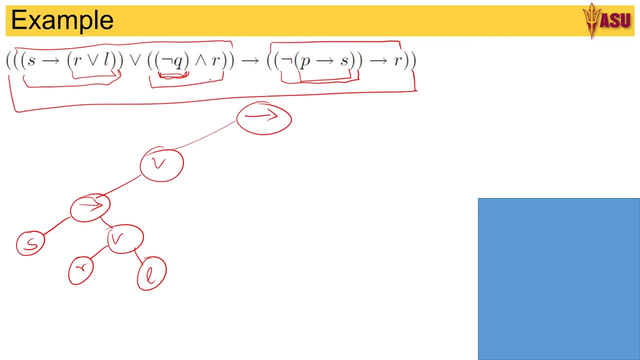 Now I have to come back one step higher, which comes to the R and over here. The R has an AND over here. Okay. 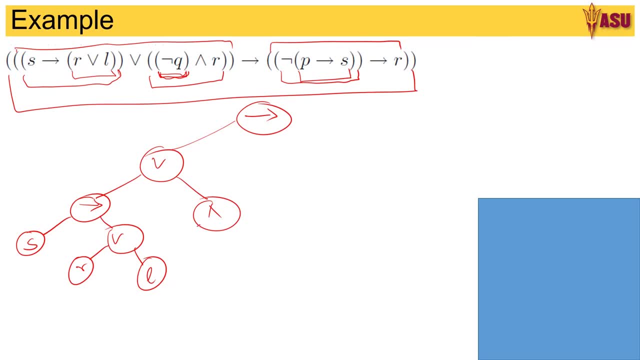 So I have an AND over here, followed by a NOT Q to its left and then R to its right. So this completes this entire part of the formula. Now I have to move to the right side of the implication. The right side of the implication, again if you look at this formula, the implication forms the center of that formula. 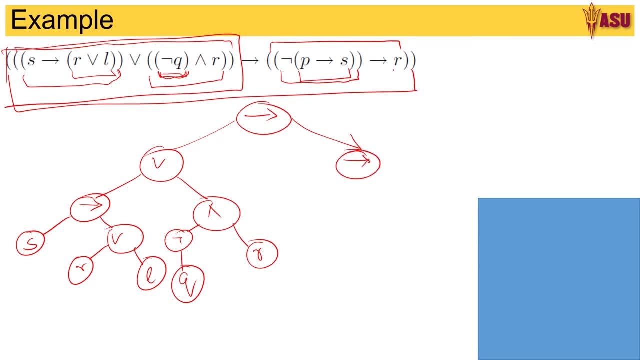 So I get an implication. To the left of the implication is this entire formula and it has a NOT on the top. 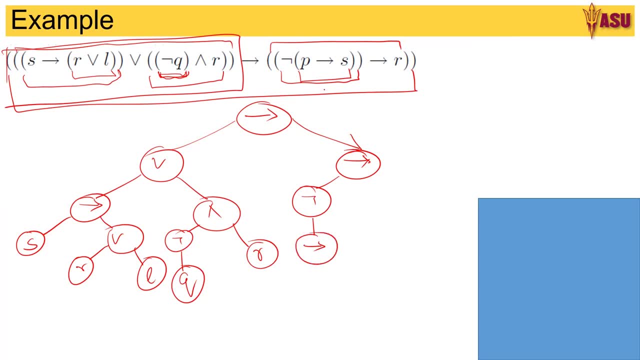 Again the NOT has an implication. Remember NOTs are urinary operators, while the others are binary operators. And the implication has a P to its left and S to its right. And this completes the left of the second implication. Okay. Okay. So this completes the left of the second implication and to the right is an R. 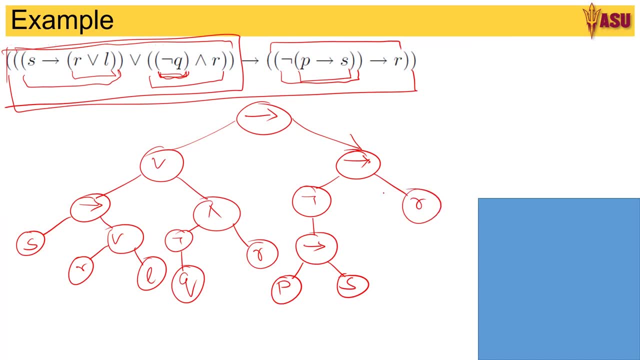 So this forms the entire parse tree for the above formula. 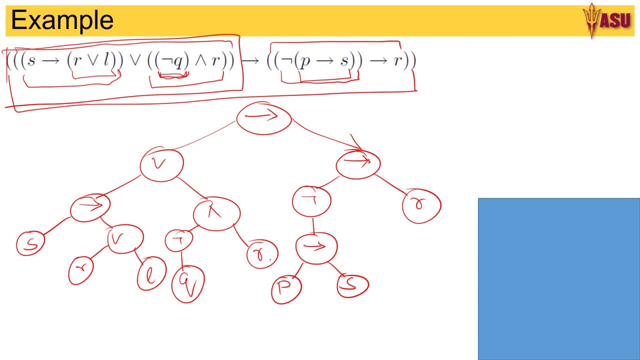 Now what are subformulas? So look at what all are there in the leaf nodes. 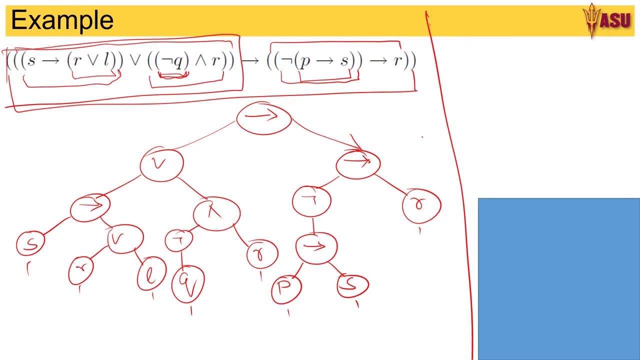 So I'm going to write the subformulas here. So I have P. Okay. 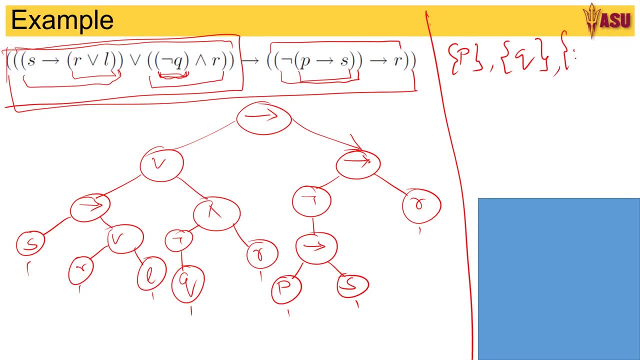 U, R, S. So I have taken S. I have taken R, L. L is remaining. So that makes a L. So that completes my leaf node subformulas. 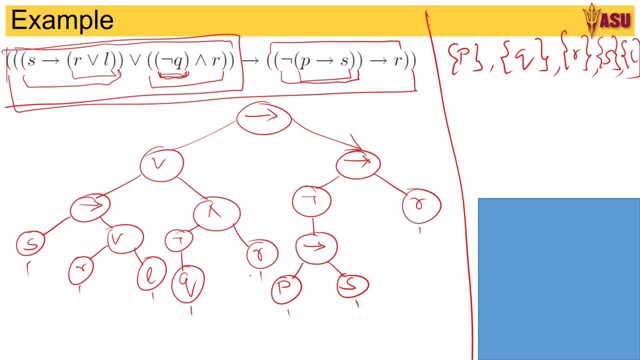 The next level. Is there any negations is what I will look at. 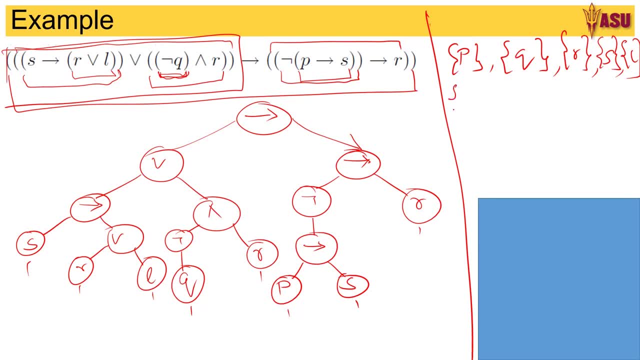 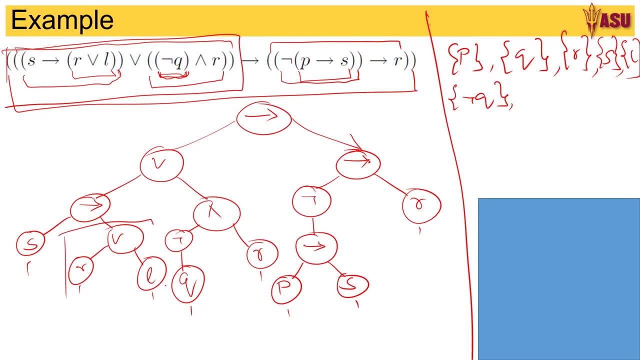 Then the next level. The next level would be this sub-tree. This sub-tree. So taking these two, I would get R or L. The other one will be P implies S. Right. Now again, you see, a NOT above P implies 3. 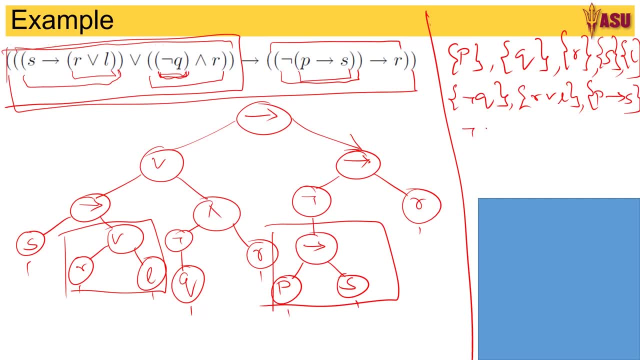 Okay. above p implies s. So there is a not of p implies s which is another subformula. Now 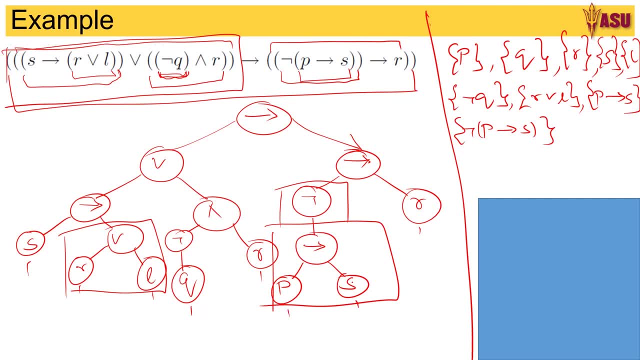 this completes this level. Now to the next level would be this formula, this formula. 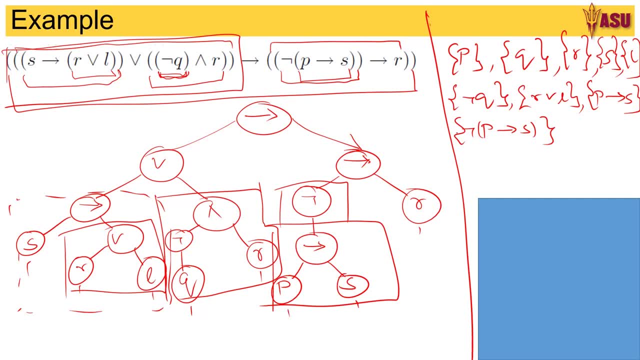 These two, taking these two, we get s implies in bracket r over l. The other subformula we get is not q and r. Ok. So this completes the next level. Now we have the one level below. 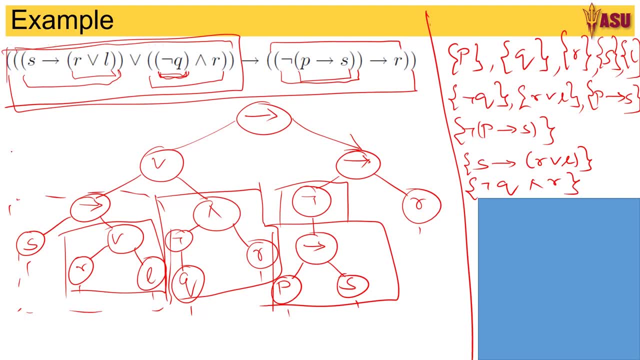 So that is this and this. So what are the two formulas then? Here we have s implies r over l, putting another bracket over here, and r. 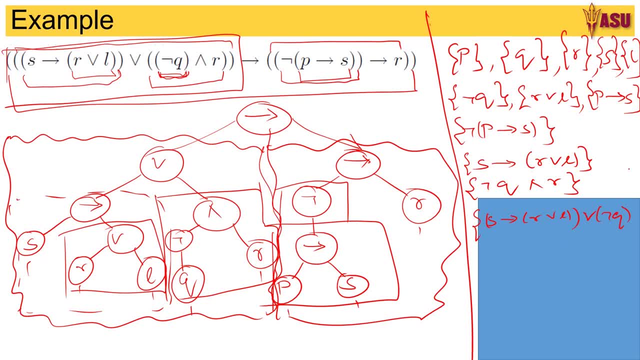 Bracket open, not q. Bracket open, not q, and r. In bracket again. So this is one subformula. And the second subformula will be from here and here, which is not of p implies s over l, implies r. So that completes all the subformulas over here. I suppose that's quite simple to do once you have the parse tree and the equation that's given for the parse tree. Remember 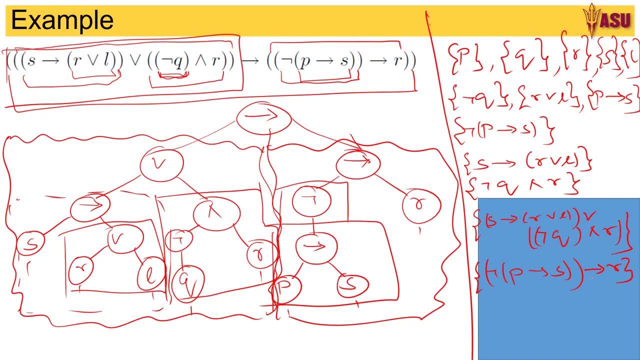 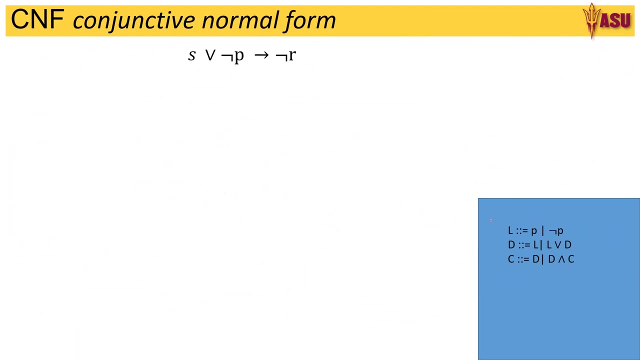 you should be able to convert both ways, from a parse tree to an equation, to a formula and a formula to a parse tree. Both these are required when you are doing these examples. Now as another part to this let's see what do we mean by c and f. c and f, the definition of c and f gives these three statements that there is an atom or not an atom. And then you have r of an atom and a formula. A formula d can either be the atom or r of the atom 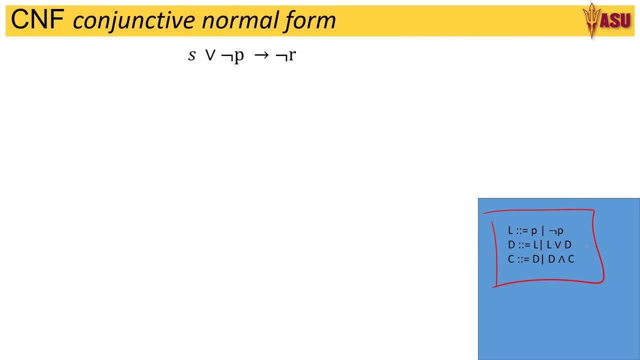 with a formula. And the second part is the formula of the atom or not the formula. So a formula can be d conjunction d d and d so in a simple manner it is 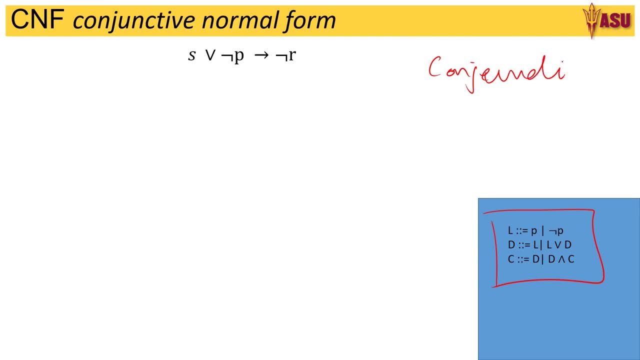 conjunction of disjunctions 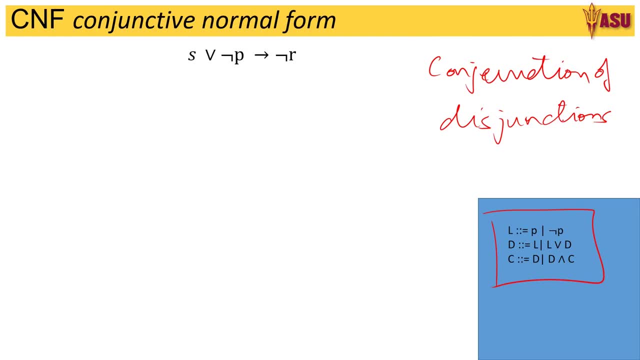 that's what is the way i remember easily what what's a cnf so to convert this formula to a cnf what do i do the first thing is i have to replace things like implications with their appropriate 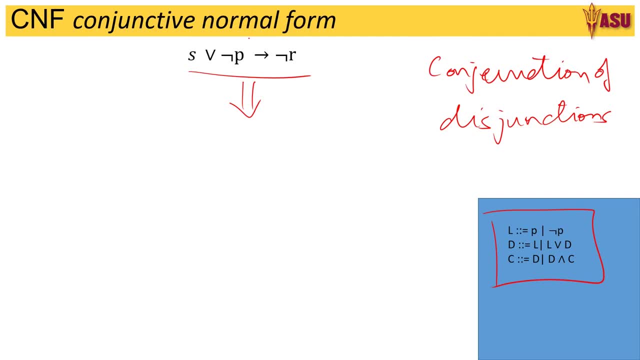 or or and formula okay so what's how can we write not p implies not r in terms of or or in terms of and the simplest way to write it in terms of r is not p implies not r is equivalent to not of not p or not r now this will become not of not will become p so that is p or not r so this is the formula right so this will give replacing this in the above formula we get s or p or not r now is this in cnf form 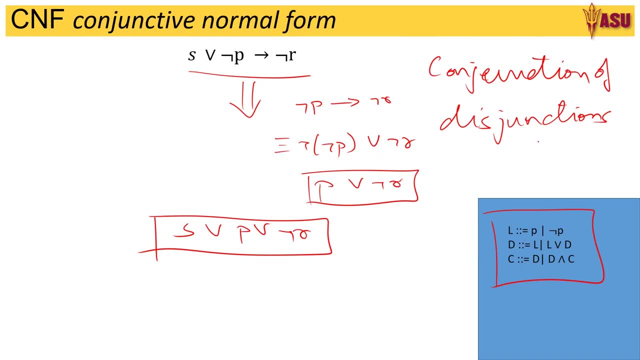 yes because the final conclusion is disjunctions over here okay and there are no conjunctions 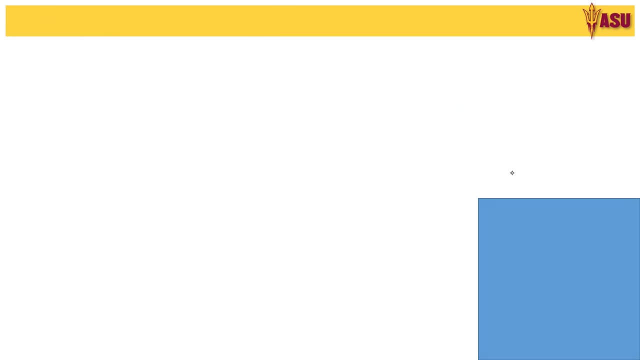 so the distribution is correct let's look at another formula for converting into cnf so let me take this formula of not p and q 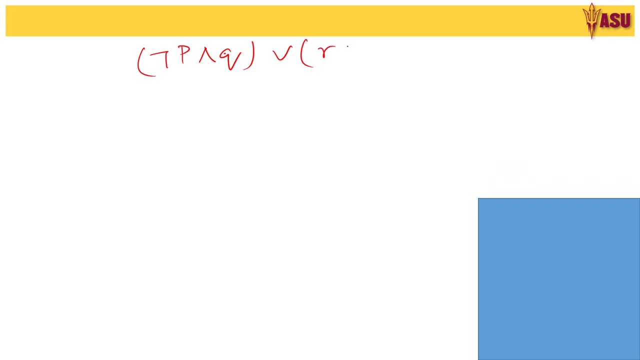 or r and s so remember uh i'll have to distribute the disjunctions to get conjunction of disjunctions that's the way cnf is so spreading using the distributive law i get this is equivalent to not p or r and s and q or r and s again applying the distributive law once more this would give rise to not p or r and not p or s and q or r